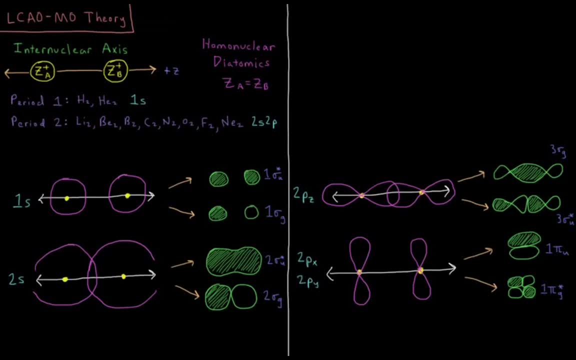 This video will discuss the idea of the linear combination of atomic orbitals to form molecular orbitals- theory for producing molecular orbitals. So we're going to start with some diatomic molecule. here. We're particularly interested in homonuclear diatomics, diatomics where each 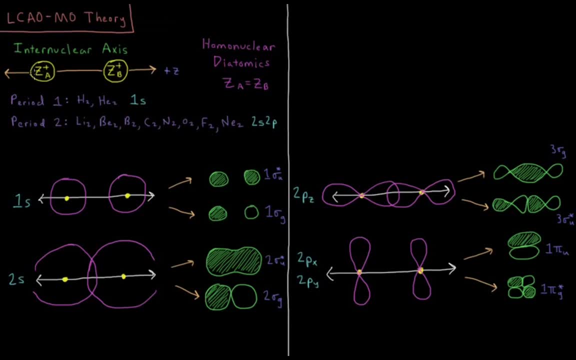 nucleus is the same. So we have nucleus 1 with charge z a plus. It has z a number of protons in its nucleus. Nucleus 2, z b plus for a homonuclear diatomic. z a equals z b Those. 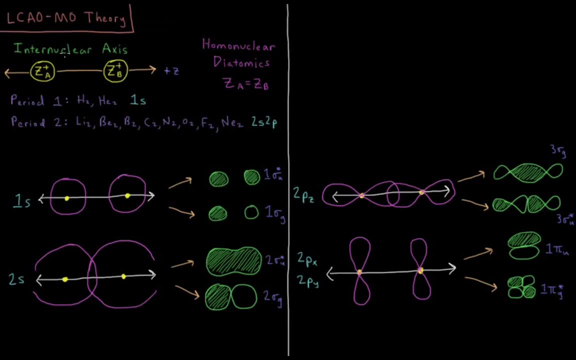 are both arranged on the z-axis, which is the inter-nuclear axis, the axis between our two nuclei. So what we're interested in is building up what the molecular orbitals are going to be for our period 1 and period 2- homonuclear diatomics. So that includes the H2 molecule. 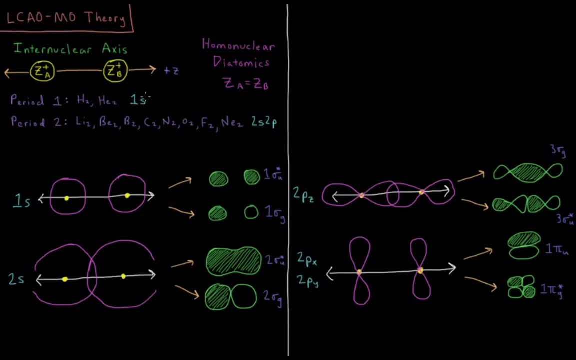 helium 2, things that involve the valence shell of having a 1s, and then lithium 2, beryllium 2, boron 2, carbon 2, nitrogen 2, oxygen 2,, fluorine 2, and neon 2.. The period 2 having a valence shell of 2s. 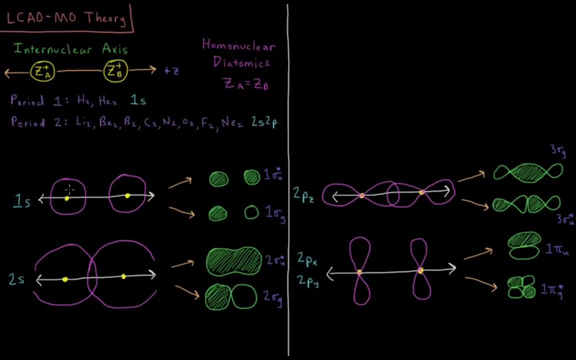 and 2p orbitals. So, very simply, the idea of LCAOMO is that these atomic orbitals are going to combine. so linear combination just meaning that you're adding them together. Atomic orbitals, meaning our basis set are going to be the. 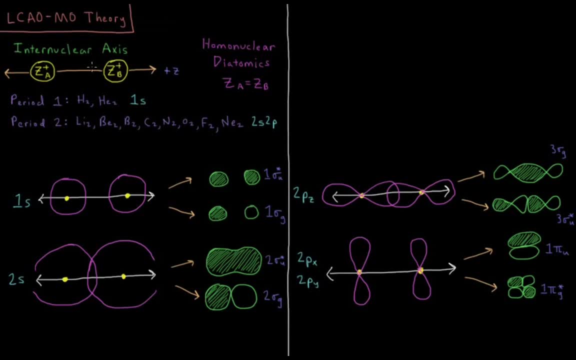 atomic orbitals of each of these individual atoms in this diatomic And then molecular orbitals, This linear combination of our atomic orbitals is going to form the resulting molecular orbitals. So quite simple and qualitative terms. So 1s orbitals are going to overlap. 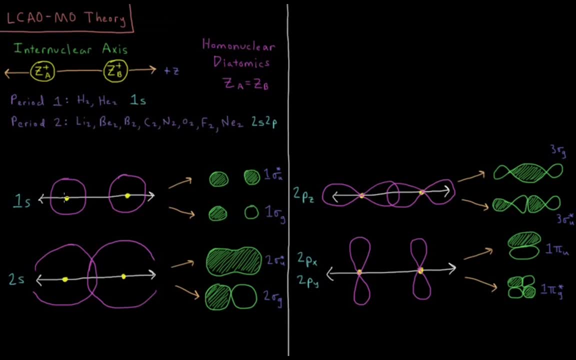 Those will form our lowest energy orbitals because they're the lowest energy states: 1 sigma g and 1 sigma u star. So these are both sigma orbitals. They're cylindrically symmetric down the internuclear axis. I have them mislabeled with respect to Gerada and Ungerada, so let me 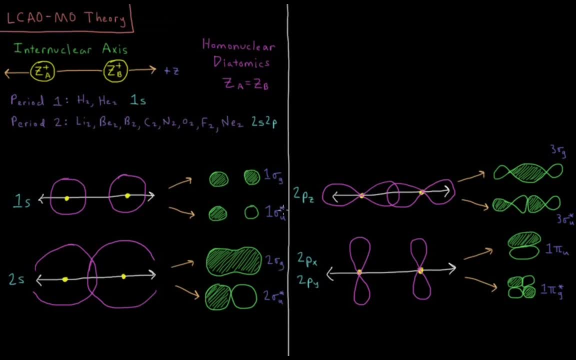 fix that right now, Much better. I also had the stars messed up. Okay, so we have the positive overlap of 1s orbitals leading to our lowest energy, sigma g orbital. This is symmetric with respect to inversion, It's a Gerada orbital. so 1 sigma g bonding, We have the antisymmetric.